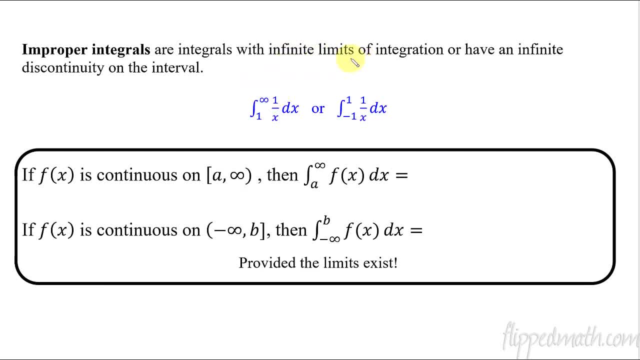 we are going to have either an infinite limit, so either the lower limit or the upper limit is an infinity, or maybe even both of them, or somewhere within the interval from negative one to one you have a discontinuity. that's an infinite discontinuity, like a vertical asymptote. 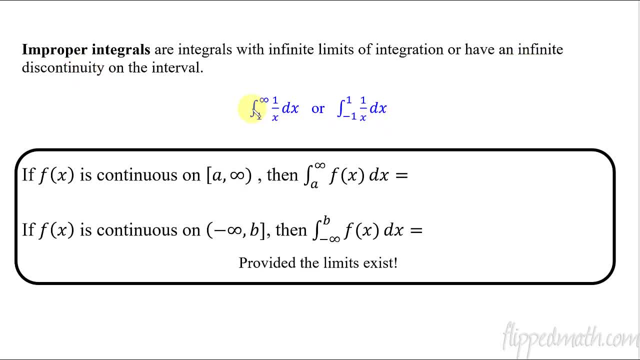 Okay, so infinite discontinuity inside that interval, that's what we have. when we have one of those situations, we have what's considered an improper integral. Well, those are a little bit more difficult to evaluate, because we're going from infinity to infinity and we're going forever here, Like: can you even figure out what it's? 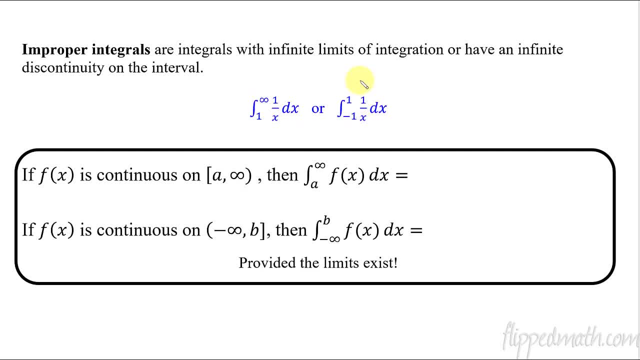 what the integral area under a curve is. if you're going forever, Well, sometimes you can and sometimes you can't, and so we'll talk about the difference between those in here in just a minute. So let's start off with: if we're going from a to infinity, so we have a continuous function f, we're just. 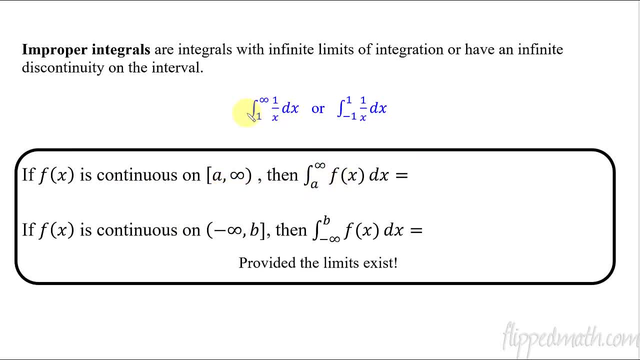 going to go from a to infinity. How do we do this? How do we evaluate that if we have an example like this one right here? Well, this is what it looks like: we're going to use a limit, and the limit is we're going to replace the infinity here. 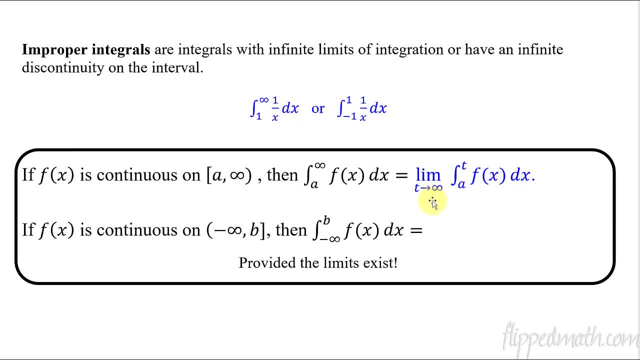 So we're just saying an upper limit of infinity, we'll put in a t and then just say: have a limit as t approaches infinity. You see, we can't really evaluate an integral plugging in an infinity, but we can say we're going to approach infinity. so that's the only difference here. And then this one: if we're 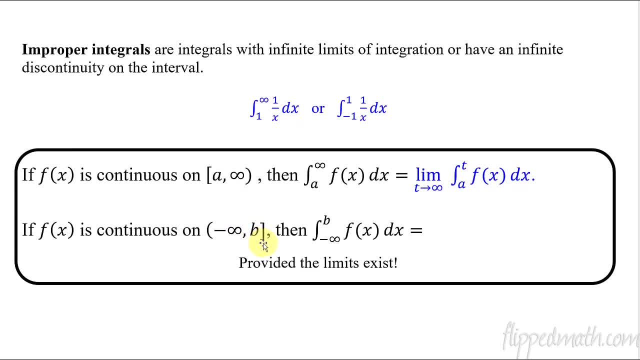 going from negative infinity up until some included value. notice that the b is included, same up here the a was included so that lower limit was part of it, part of the function. So here the b is in the domain of the function and we're going up until b. so 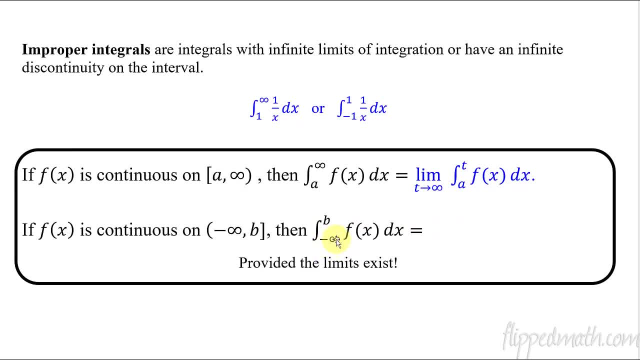 it's. hopefully you can kind of figure out what we're doing here. If we're going from negative infinity to b, what would this be The limit as t approaches negative infinity? and then we're going to go from t- this time is on bottom- from t to b, because the negative infinity is getting replaced. 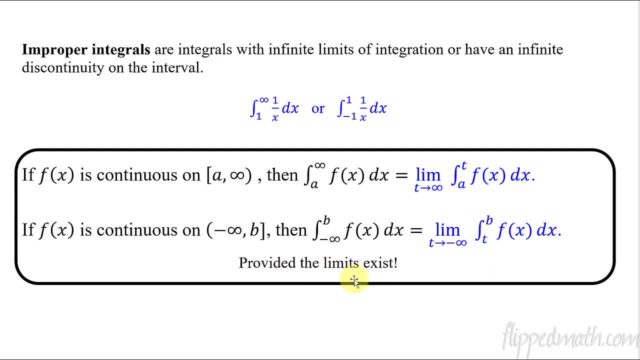 with substituting in a t value. Now, this only works if the limit exists. so provided that these limits exist, then this statement holds true. If the limit doesn't exist, then we're not going to be able to evaluate the integral. You won't be able to know if the limit exists or not. 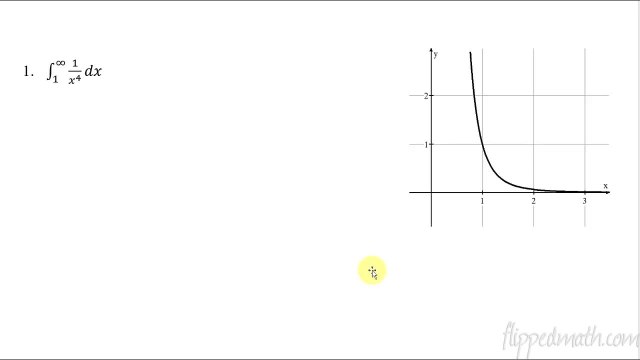 It doesn't actually go to one specific number. We'll talk about what that means here on our next slide after this one. So let's practice with what we have learned so far, and that is, if we're finding the area under the curve from one to infinity, that means we're doing this. So just 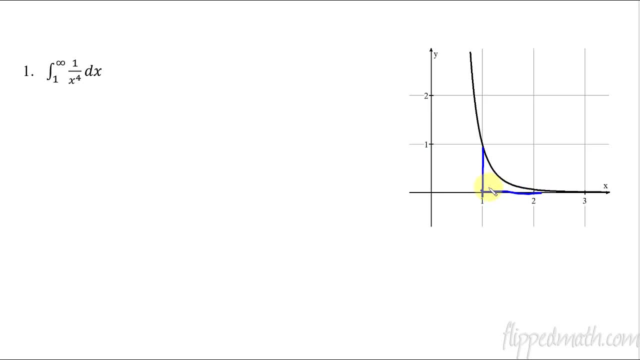 what's the concept here? we're going from one all the way to infinity, so we're doing the area under the curve and we just keep going and going and going. but notice, the area gets really, really tiny right away. it gets small by the time we're three. it looks like it's already there. It's not, if you. 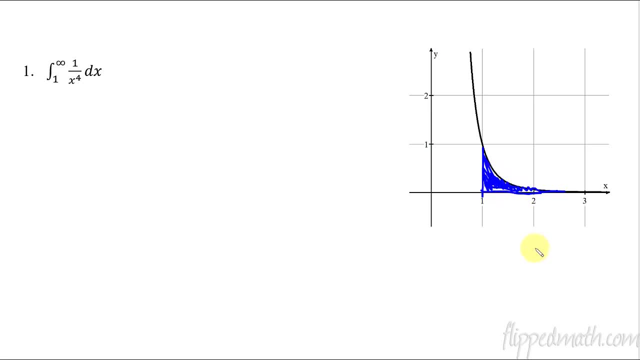 're? I mean, it's not going to be zero, but it's going to be awfully close. so does this approach a specific number, that area? well, let's find out. we first rewrite this as the limit as t approaches infinity of, and now we do our integral from 1 to t instead of to infinity, and then I'm just going. 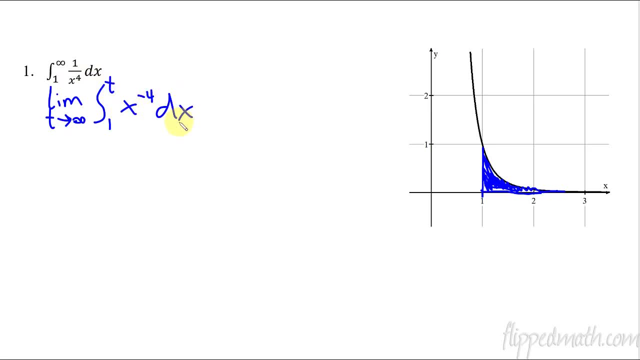 to rewrite this as x to the negative, 4 with respect to x, and that'll help me a little bit when I'm, uh, anti-derivating derivative, whatever, taking the anti-derivative and then what's this going to be here? so we take the anti-derivative. I. 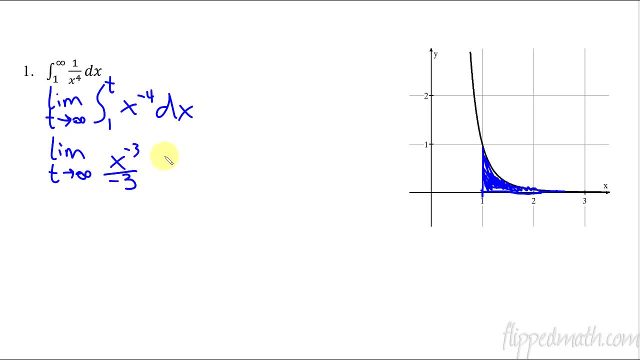 get x to the negative 3 divided by negative 3, and I'm evaluating it from 1 to t. so now we plug in the t so limit as t approaches infinity- and yes, it gets tedious writing this limit down all the time- so this is now going to become plug in the t first and we get negative 1 over 3, t cubed minus. 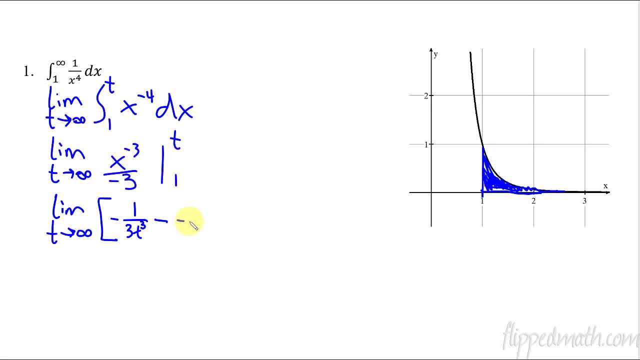 and now we plug the 1 into this, so we still have the negative. so it's going to be a negative 1 over 3, 1 cubed, all right. now, what does this equal? well, now we are going to have t approach infinity, and that's. 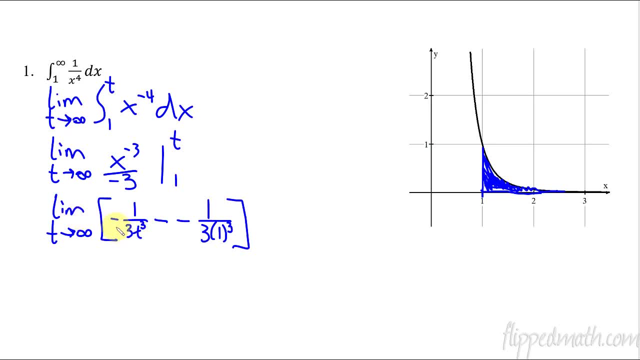 where we use the limit. so as this t approaches infinity, that whole fraction here gets closer and closer and closer to zero. so this just becomes zero plus 1 over 3, or in other words this equals 1, 3.. so this area here is going to a very specific number of 1. 3rd, and what we do: 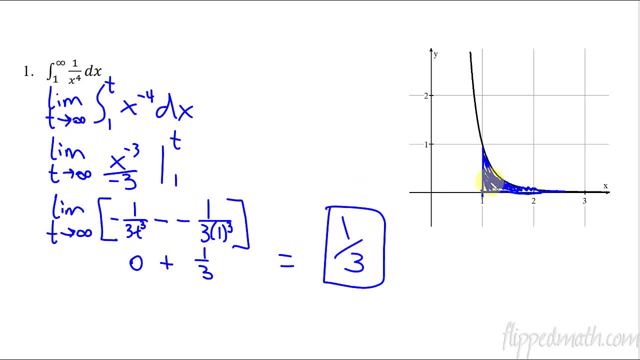 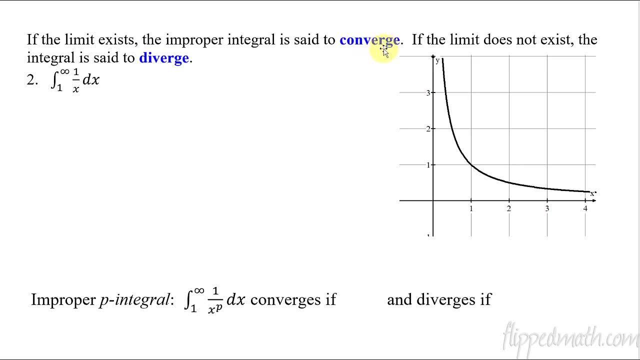 is. we say that it converges to 1, 3rd. that's what this area is going to be as you go more and more and more off to the right infinity. so that leads us to some new vocabulary and that is converging and diverging. so we, you, some of you may 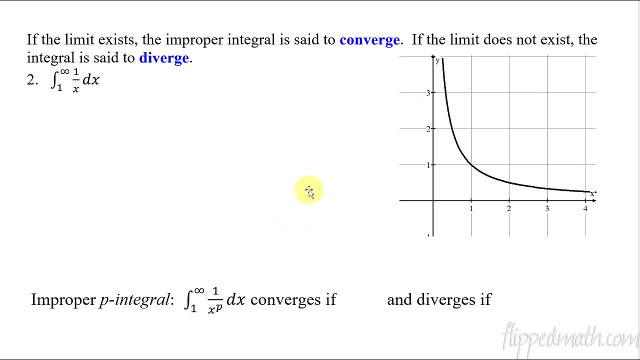 have had this in pre-calculus. it just depends on what course you had, maybe what book you use, whether you studied these two things- convergence and divergence- and it's not those movies that's which we're not very good. so if it converges, we're saying that the improper integral is going to a very 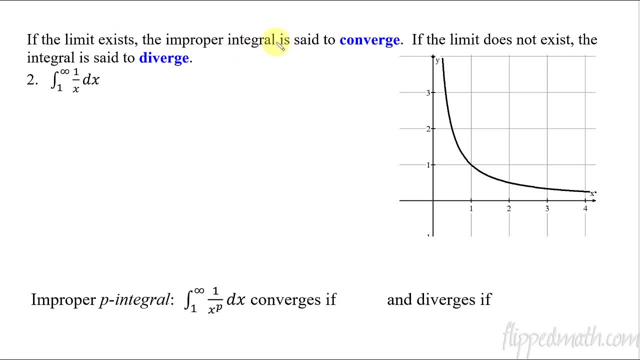 specific number. so if the limit exists, then the improper integral is converging to a number, like in our last example: it, we, it converged to the number 1. 3rd, if the limit does not exist. so if we are working through this limit and we find 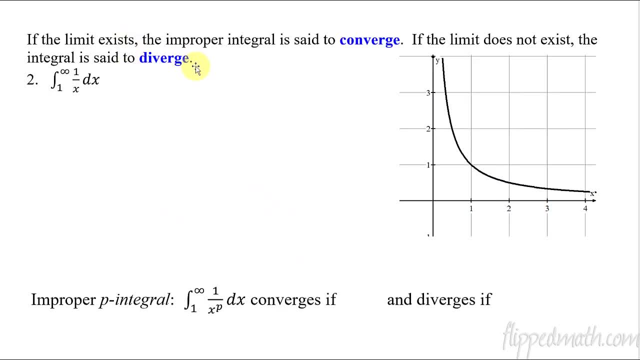 that the limit doesn't even exist. then the integral is said to diverge and we're not growing towards a specific number. the area doesn't converge to a number, it diverges. okay. so here's an example of something diverging. so let's see how we set this up. notice here. so I'm the idea. 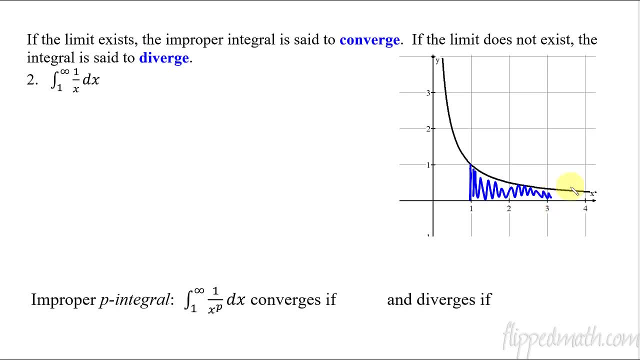 is, we're taking this area. so you'd think, as you, as the area, you just kind of keep going, if we stretch this off, way off to the right, it would get really really close to zero, right? you'd think, okay, well, doesn't that converge? but you 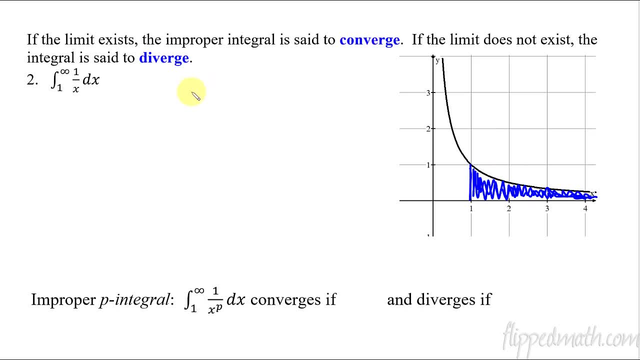 cannot just use the graph and make a determination on if it converges the diverges. you have to work through the mathematics and trust your answer there with these rules, Not just looking at the graph and assuming that it converges. So let's do the limit as 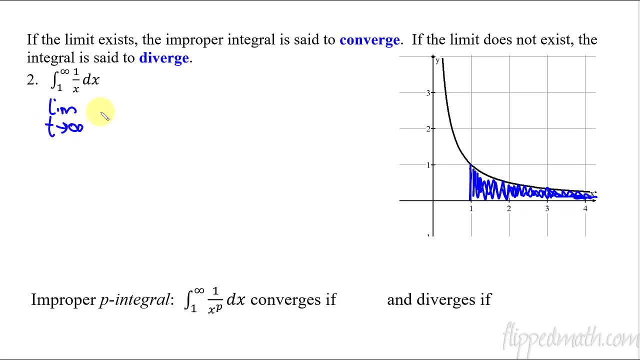 T approaches infinity, and this time it's going to be- what do we have here? the integral from 1 to T, of 1 over X, DX, and then the next step down will be that the limit as T approaches infinity, of Now this is going to be the natural log of absolute value of X and evaluating it from 1 to T. 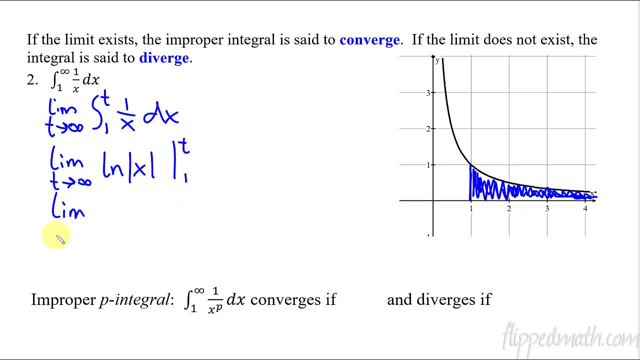 So the T gets plugged in first, although I still have to have my limit here, my limit as T approaches infinity. So now I'm going to have the natural log of T, absolute value of T minus the natural log of 1. as T approaches infinity, This natural log of super large number is still gonna approach infinity. This is just going off to infinity. 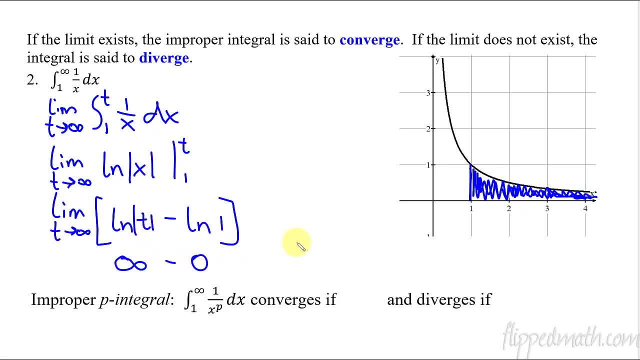 Minus natural log of 1 is 0, so that one's easy. But this is approaching infinity and that's why it diverges. It does not go to a very specific number. So that is an example of something diverging when the limit doesn't exist. 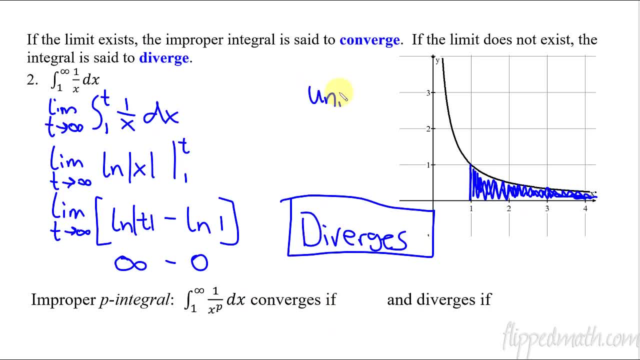 It just goes off to infinity like that. when we get to unit 10- Our very last unit of the year for BC calculus- when we get to unit 10, We're gonna talk a lot more about convergence and divergence with series and, in particular, this stuff here with us, these weird things going on. 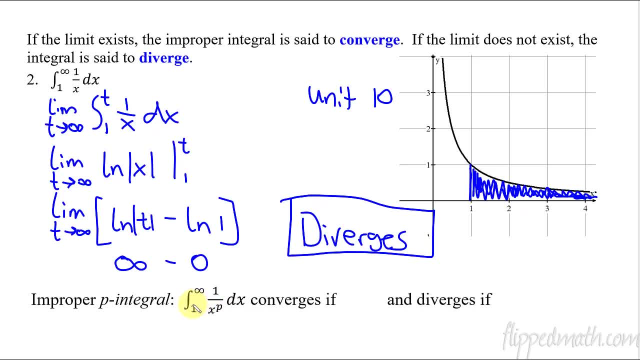 Here. this is something that I want to make sure you understand, and that is when you have this situation: 1 to infinity with 1 over X to the something power. So we just did 1 over X to the first power. the example before was 1 over X to the fourth power. 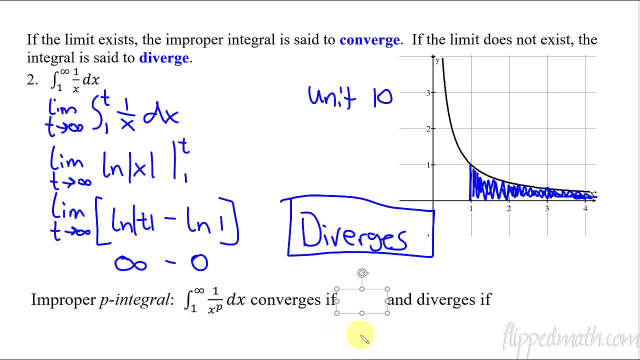 so when that power, P, is Larger than 1, it converges. So if you ever have 1 over X to the number that is larger than 1, it's converging. if it is Less than or equal to 1, then it is diverging that power right there: 1 over X to P. 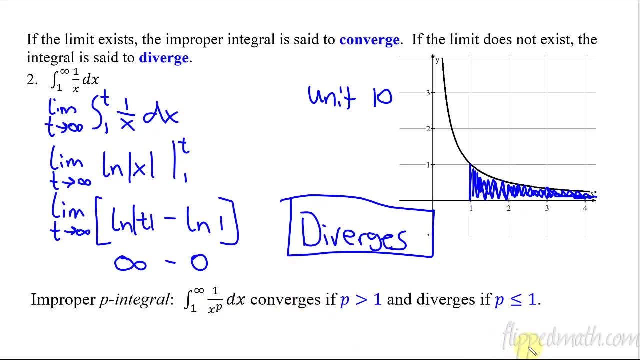 So that's kind of an important one to remember. we will that. it will pop up a couple times here and there and we'll have a little bit of that in the practice as well. Okay, this slide, lots of different words on this thing, hope, much of words. 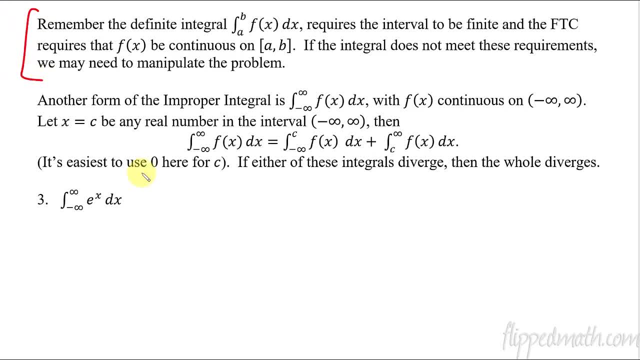 This first paragraph here is just reminding you something that we've already talked about, Okay, so just reminding you that this has to be a finite interval and That the fundamental theorem of calculus States that F of X has to be continuous. So what we've been we're gonna work with is situations where that doesn't happen. 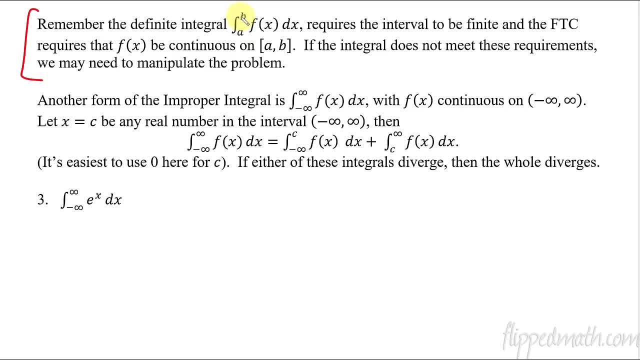 So where we already did, where a or B, could it be infinite infinity? right, it's going off to infinity, So it's not a finite interval. So we had to use a limit to help us understand how to work with that. And then we're gonna talk about a situation where f of X might not be continuous. 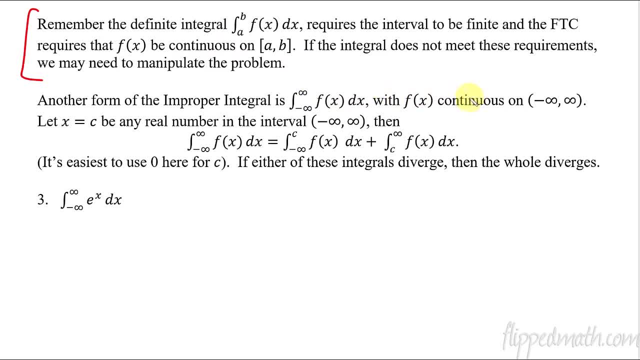 So we're gonna see if there's a way to still solve it that way. So if f of X is continuous- So right here we're continuous from negative infinity to infinity- Then C can be a number in the interval, any real number that we're allowed to just split it up. 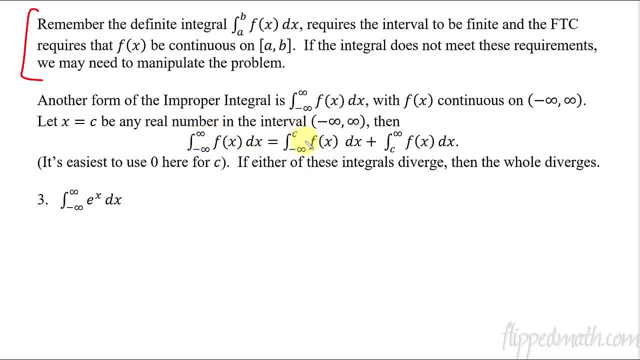 So look at this: if I go from negative infinity to infinity of f, of X, I could split this up and go negative infinity to C and then add the integral from C to infinity. Okay, that's just our rules that we worked with with the properties of integrals. 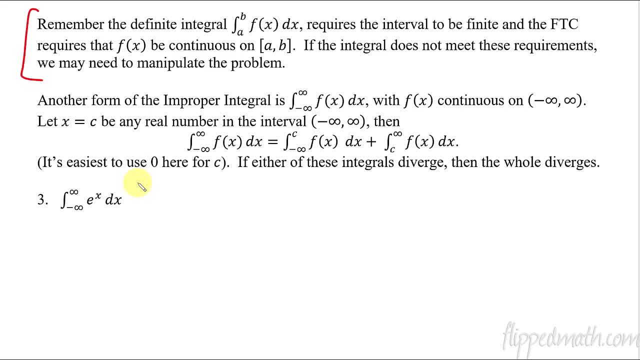 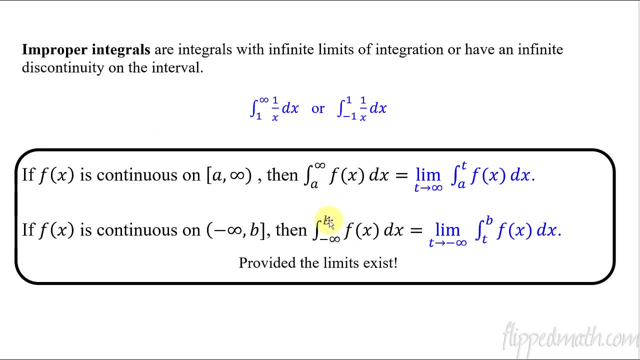 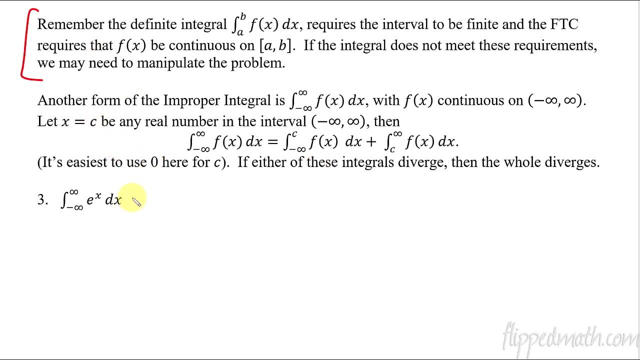 So the reason we want to do that is so that then we can use this right here. You can go from negative infinity to a number and then that same number will use the same number and off to infinity That number that I would choose. I would always use zero because it makes it really easy. So this equals: 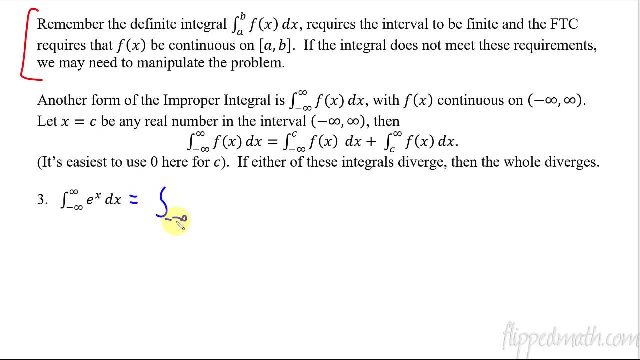 We're going to do the integral from negative infinity to zero. and then what are we doing? e to the X, with respect to X plus. Now we'll go from zero- the same number, So zero is my chosen C- to infinity, of E to the X, DX. now, we can't use infinity to do these integrals. 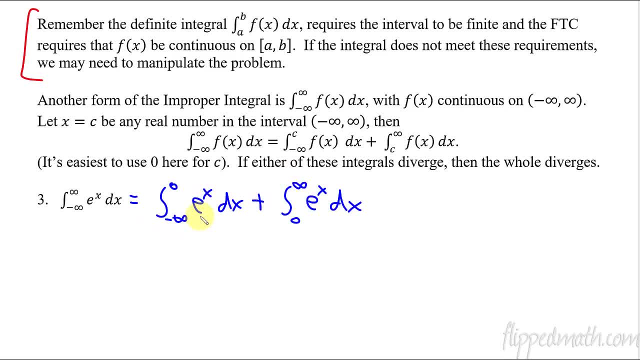 So that's where we're gonna use a limit, but the limit is difference. We have two different integrals here that we're using a limit for, so for the first one We're gonna say the limit as T approaches negative infinity, and then we'll go from T to zero of. 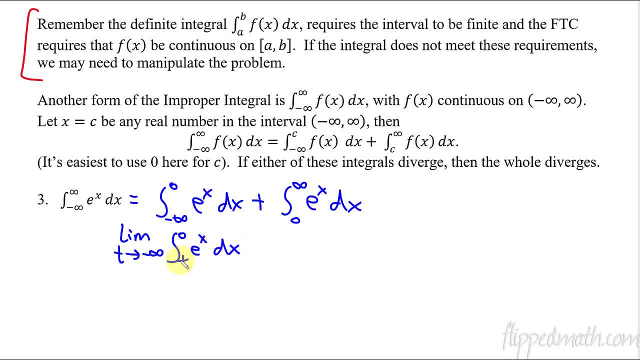 E to the X, DX. Sorry, that's getting a little sloppy. That looks like a four. That is a T right there, Not a four T Plus. and now this has an infinity within the integral, So we have to change this and make it a limit. 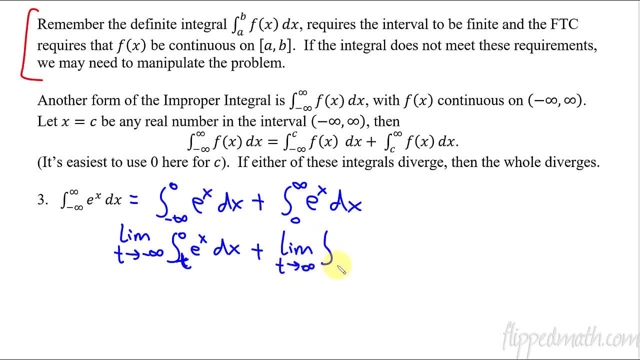 So we're gonna say: the limit is T approaches infinity, and then we'll say: from zero to T, of E to the X, DX. So now you have two separate problems that you're working through. If either one of these diverges, then the whole thing diverges. 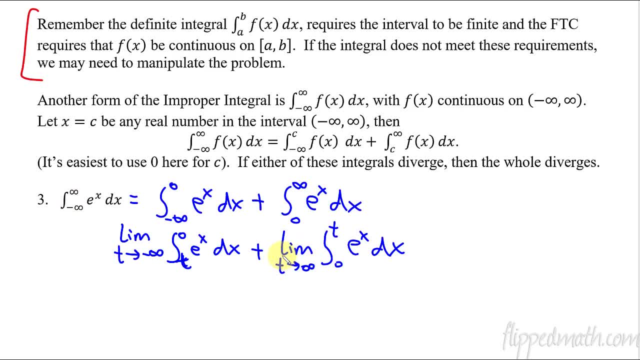 Okay. so let me repeat that if you find that one of these pieces diverges, then everything diverges, So you have to work through both of them to figure out what's going on, So you may have to pause the video. I'm gonna have this next line up here. Here it is. 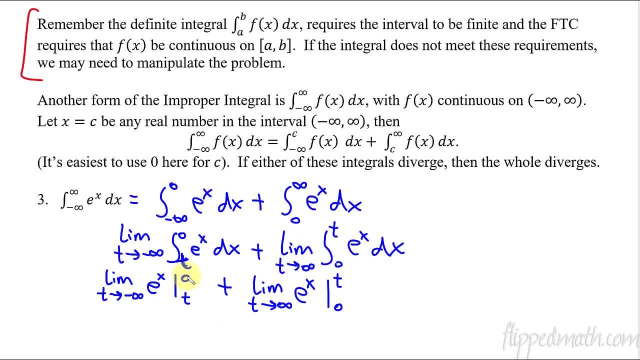 So there's my work here, and then if I go to the next line where I start plugging in some things, So again I'm gonna have this line just appear. So again you might have to pause to write that whole thing down. So this is where it gets the pretty tricky. 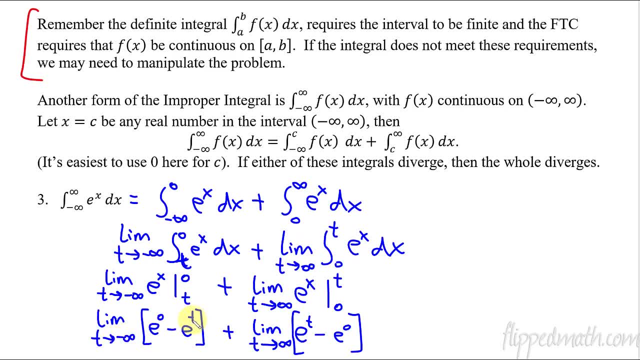 Because if you plug in a negative infinity into an exponent, see, I'm gonna, let me, let me rewrite this line up here. So if I, if I have this limit, now I take the approach with the limits: e to the zero is one, So this first part is one minus, and then here I have e to the negative infinity. 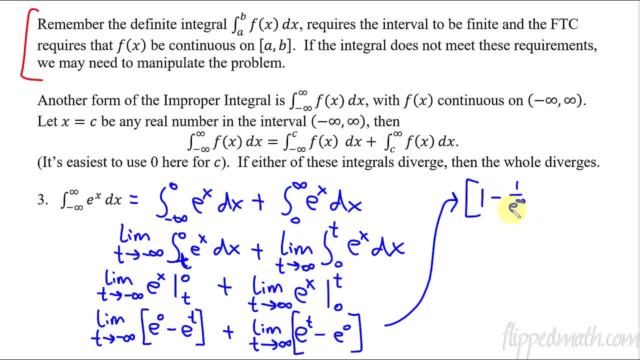 Which is equal to this e to the infinity. there, though, So this is actually zero on bottom, So I'm good to go. I can keep going here. But now the next part. I'm going to have e to the infinity, and that's the problem right here. 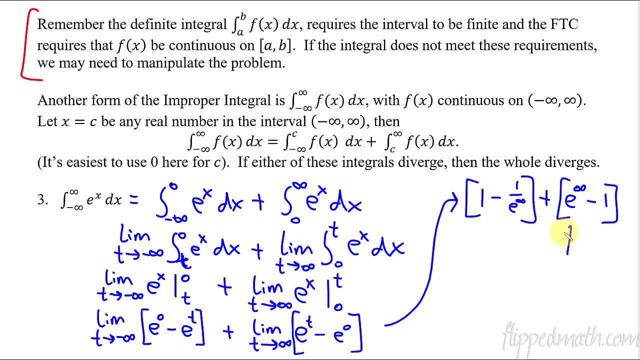 What I'm writing e to the infinity minus one. that part diverges. This is going approaching infinity. So if either of these parts diverge, then the whole thing diverges. So that's our answer for this one. So it's not. I have several examples of where it's gonna be diverging on this, on these notes. 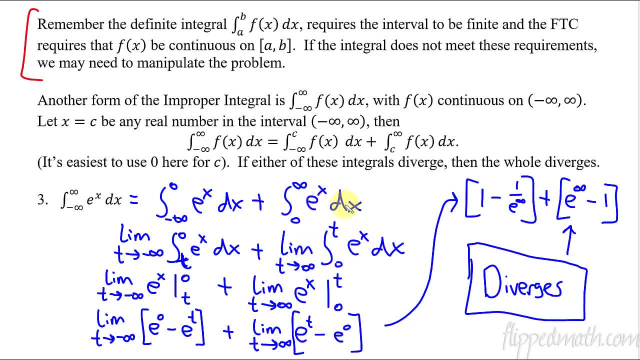 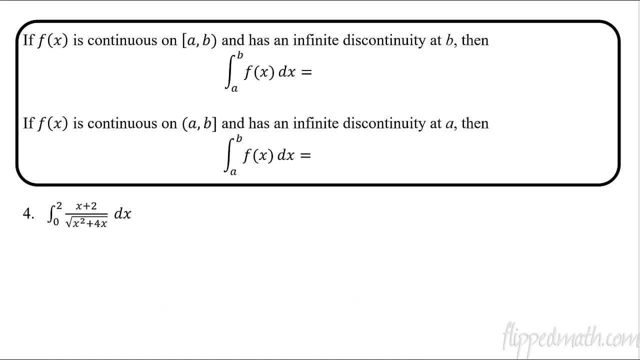 But it doesn't always. the important thing was setting up part and then going from there, and it's using things We've already been learning: taking the integral and then using your understanding of limits and how that works. All right, we're getting close. two more problems. 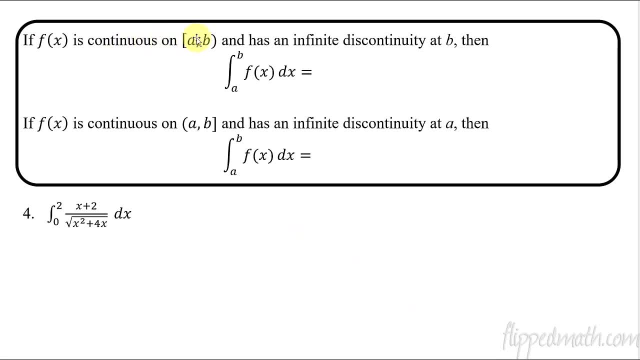 for this one. We are now going to look at a continuous function from a to B on the interval. But B- notice- here it's not including B, So it's an open interval on the end here. and that B it's open because it has an infinite discontinuity. 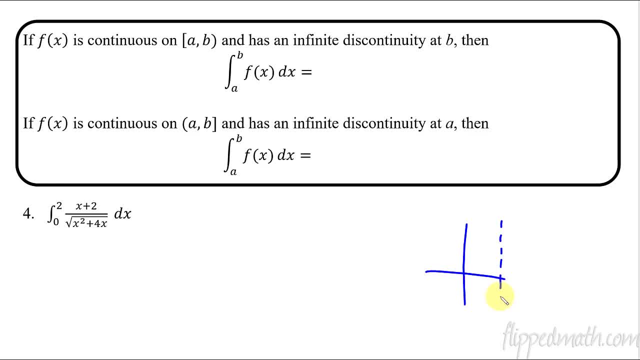 Or in other words, the graph of it. if you're looking at a graph, it's like you have a vertical asymptote. So it's approaching that vertical asymptote and maybe it peels up to the right. like that It goes up forever and ever and ever. 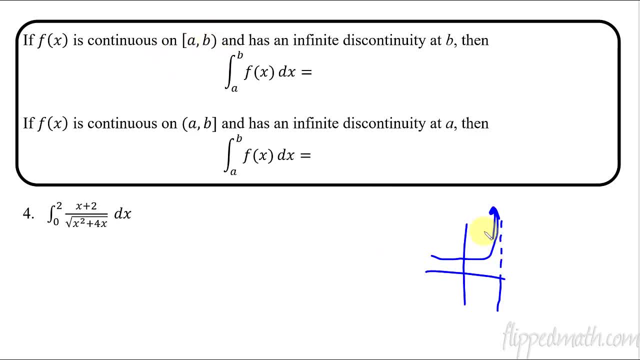 So it's a vertical asymptote, And so that's why we can't actually get to the B and include it. Okay, so that's the idea of what we're doing. So how do you do The limit when you have something like that? you do this. 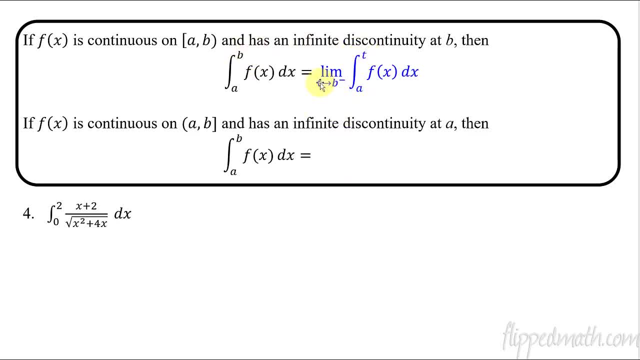 You're gonna go from B is going to be substituted with a T, and we're going to have T Approach B. Now, if you're approaching B, you have to think that you're approaching B from the left right. If you remember the picture I just drew, you're approaching B from the left side and that's why you have that. so 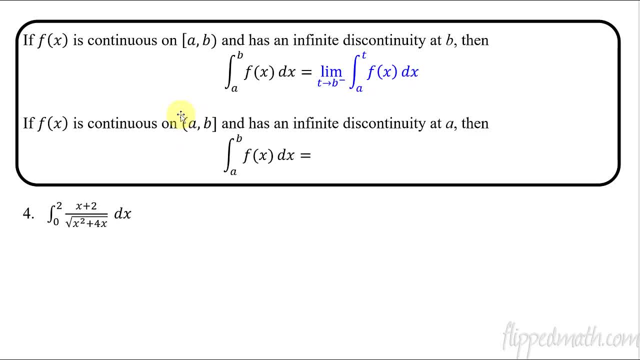 the other one if we're going from A to B, But A is the one that has the vertical asymptote, the infinite discontinuity, Then what is our limit going to be? Think through it. It's gonna be the limit as T approaches A, and then it is from the right side. 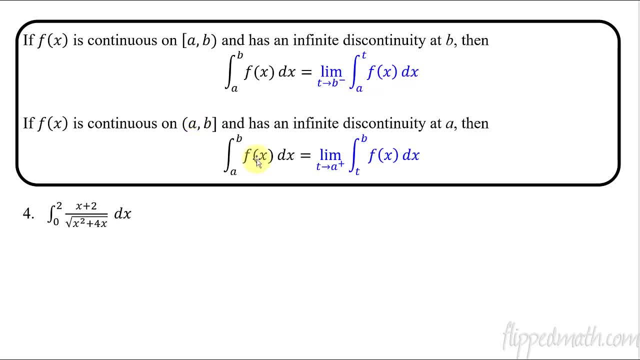 We're approaching A from the right, so we're gonna get closer and closer to A coming from the right side and working our way back, and so then A Gets substituted with our value of T, so that T can approach A. Well, I was confusing. hopefully understood that. all right, let's try this out. 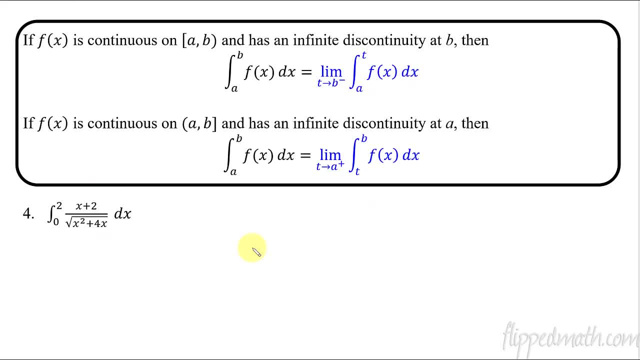 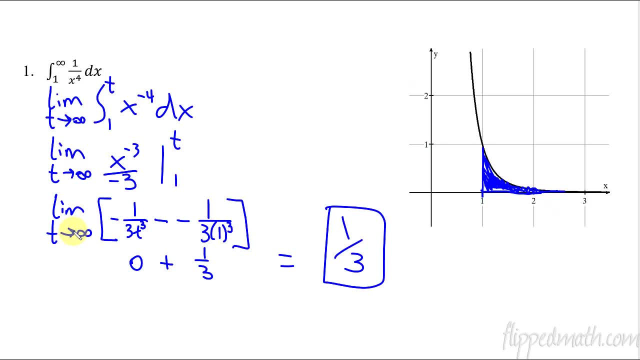 So the way you know is- and I haven't really talked about this yet, but you're supposed to always check for discontinuities. It's a pretty important thing to do. I didn't. I should have talked about this Those before. when we look back at these like our very first examples, 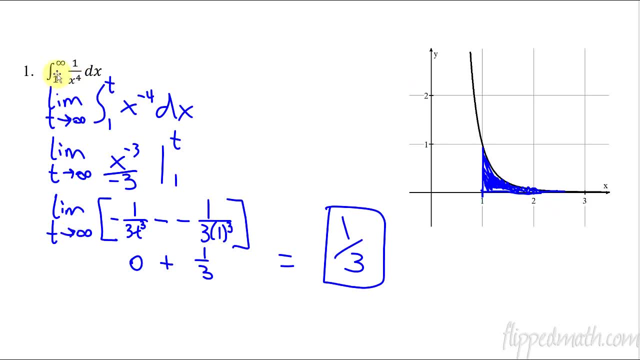 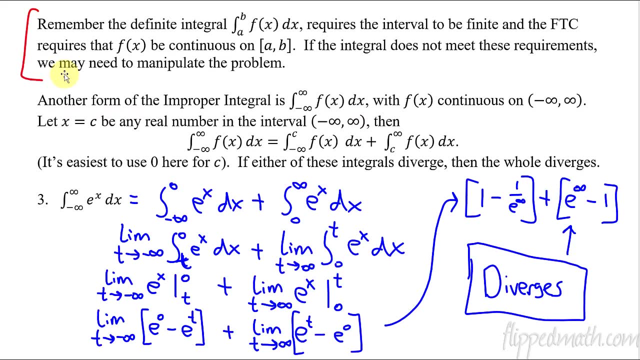 There's a discontinuity at X equals 0, but X equals 0 is not in that interval from 1 to infinity, So we didn't have to worry about it. same here: There is a discontinuity at X equals 0, but it's from 1 to infinity, So we didn't have to worry about that. Well, on this one. 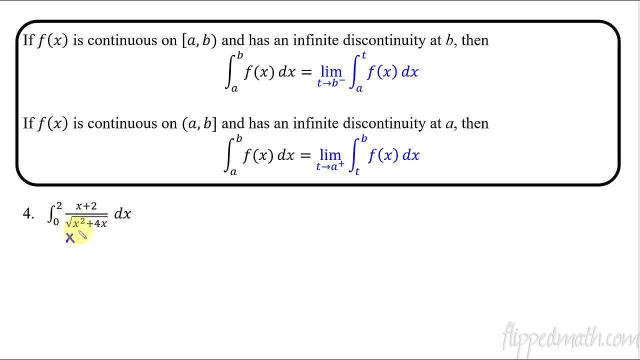 We're gonna have some discontinuities, because if I factor this, you'd have an X times X plus 4 inside that, Inside that radical. so you have two discontinuities: at X equals 0 and at X equals negative 4. Well, negative 4 is not in the interval 0 to 2, so we can ignore that one, but X equals 0. 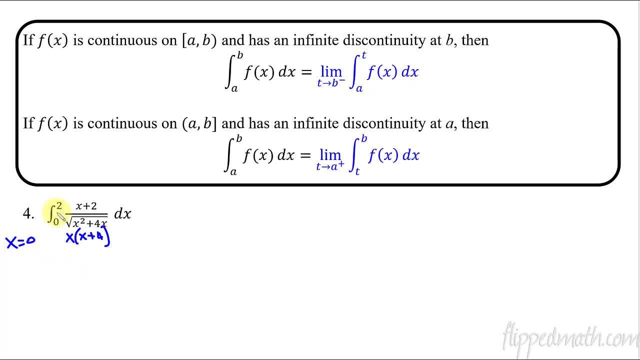 That's a problem. X equals 0, represents a discontinuity, and it happens at the beginning, so that what we're doing is we're in this situation right here. that a is the beginning and It is a vertical asymptote. It's an. it's a excuse me. 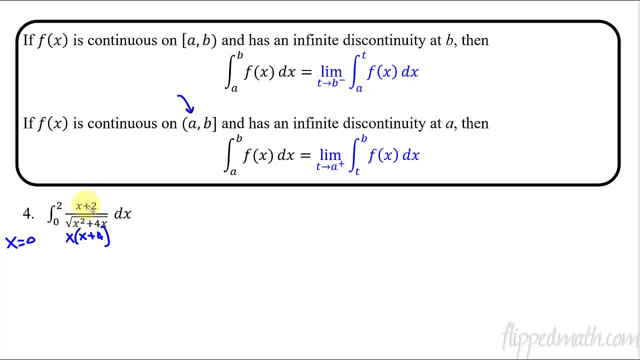 A should call it an infinite discontinuity, because it doesn't cancel at the top. All right, so let's set this up then. So this is the problem I'm working with. I'm gonna say that this is equivalent to the limit as T approaches, and this is zero from the right side, and then I have my 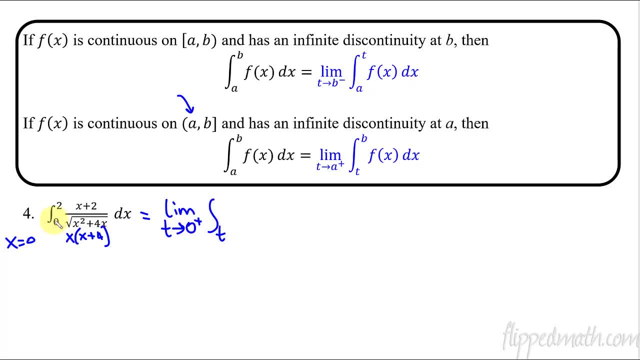 Integral here. What is it from? T? so instead of a 0, I'm going to replace it with T and I'm going up to the number 2. before I start writing this out, I want you to see That would think of heads. step ahead. how in the world are we gonna solve this crazy thing? 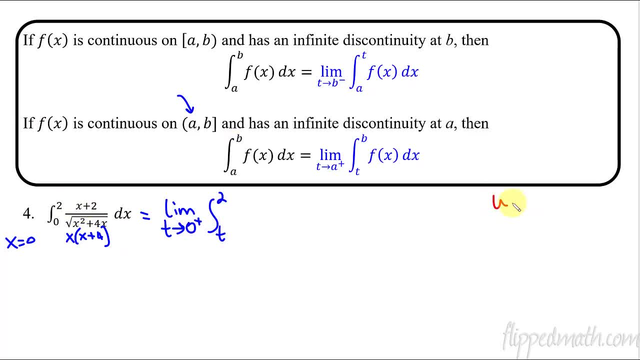 This is U substitution. Yes, it's not gonna go away. So U substitution: U is going to equal the thing on the inside here, x squared plus 4x, and then that means that du is equal to 2x plus 4 dx. 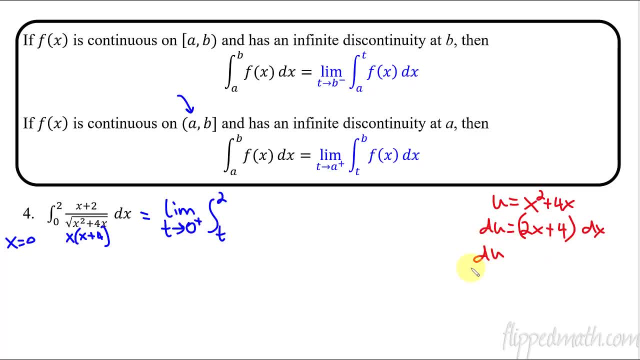 Divide both sides by the 2x plus 4, and I'm going to have du over and I'm going to factor this because I needed this x plus 2 to cancel. So if I factor this out, it's going to see 2 times x plus 2 equals dx. 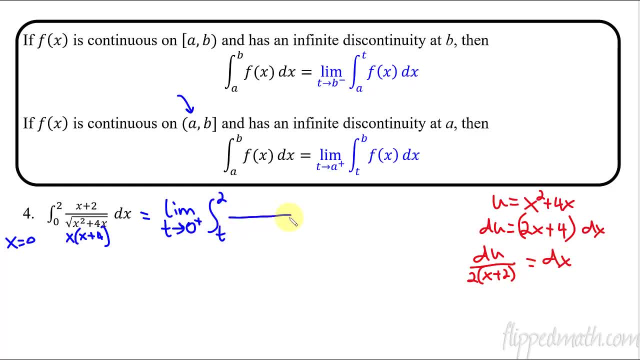 Okay, now I can start writing this out. So I'm going to have my fraction here. I still have my x plus 2 on top, but now I'll say: the square root of u, x squared plus 4x, is my u, and then the dx is going to become du. 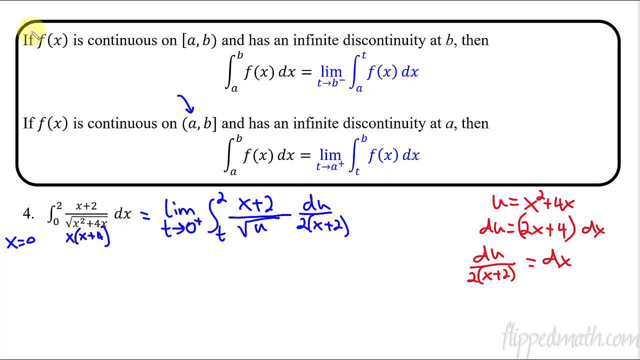 over 2 times x plus 2.. Perfect, Now that lets the x plus 2 cancel. x plus 2 cancels. and then now I haven't changed these boundaries here, right? Those haven't changed yet, so let's change those on our next step down. 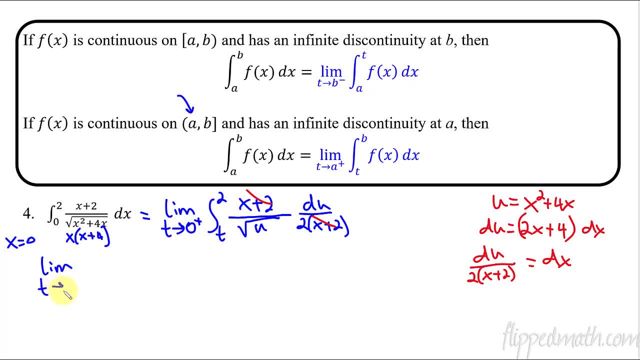 So let's write it over here: The limit As t approaches 0 to the positive- and this gets pretty tedious because you're writing this stuff over and over again- t, so the t limit. let's plug that into our equation here for u. so that's going to be t squared plus 4t, and then the upper limit of 2 gets. 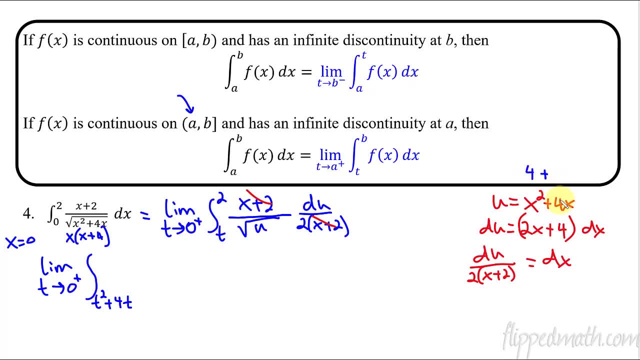 plugged in. 2 squared is 4 plus 4 times 2 is 8,. 4 plus 8,, that is 12.. Okay, big number, So 12.. And then what's important, Let's simplify this here. 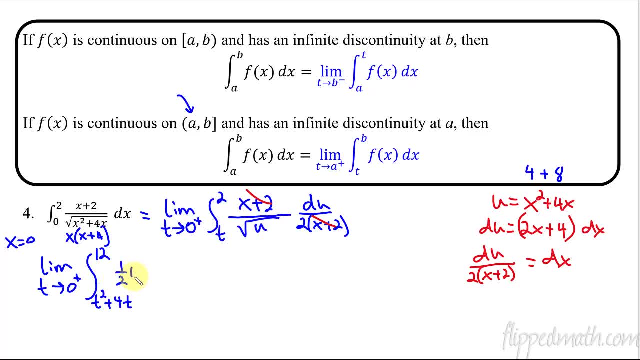 I'm going to have a 1 over 2, and then the square root of u is on bottom, so I'm going to say u to the negative 1. half du, Holy cow, all that work. we haven't even like taken the integral yet. 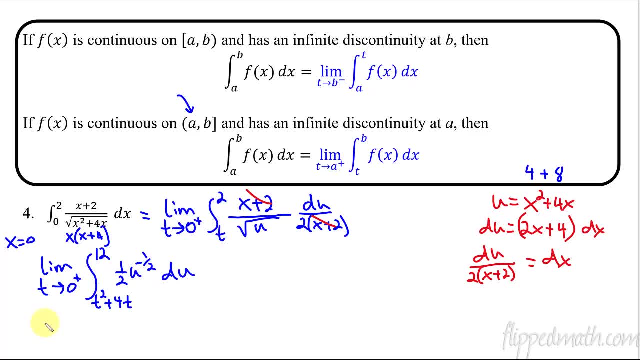 Okay, let's do this. So now I have the limit- and I do apologize, I know there's not a ton of room for you on this. The limit as t approaches 0 from the right, I'm going to pause my recording. so the answer. 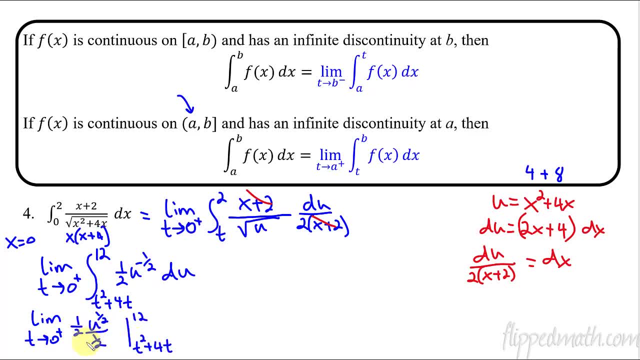 here just appears Alright. so you've got this now. Hopefully that makes sense what I'm doing here. I just wrote the added 1 and divided by that number, But that makes these 1 halves cancel. that's nice, So now I can go to. what does this equal? 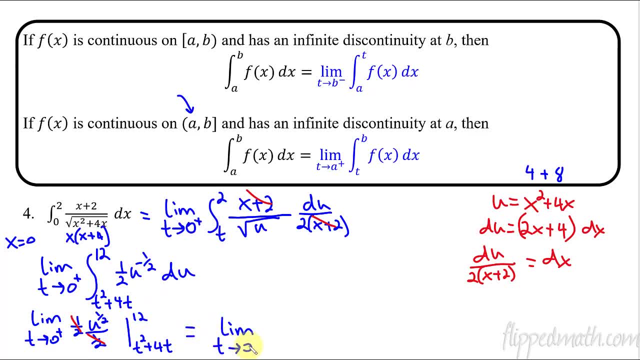 This is going to equal the limit, as t is still approaching 0 from the right side and I'm now going to have plug in the 12,, so let's do this. plug in the 12,. I have the square root of 12 minus the square root of what do I have here? 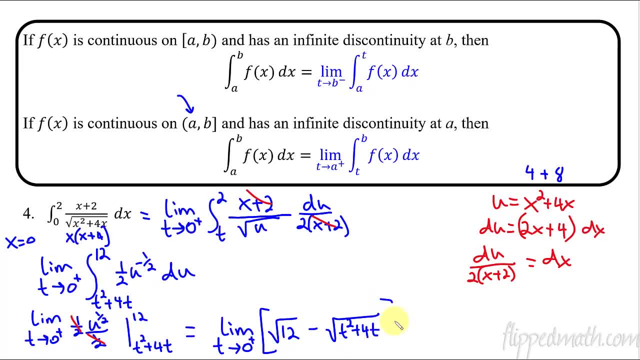 t squared plus 12.. Okay, Plus 4t, And now we have this approach, 0.. So 0 is getting really, really close to the number 0, that's what t is. so that whole thing is just 0, so it's, this whole thing equals the square root of 12, and that's our. 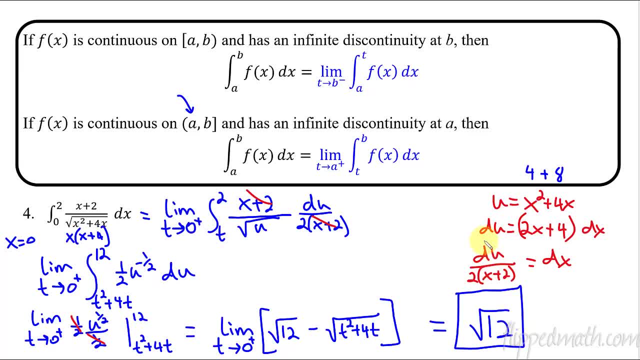 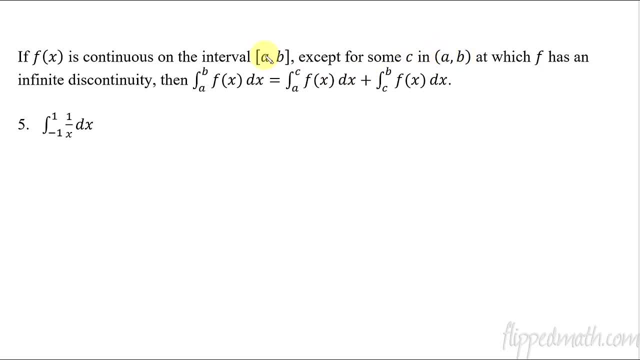 answer. So this one converges, converges to that specific number. Alright, one more example. This time we're going to have a discontinuity somewhere inside of a and b. So we're going from a to b and inside the interval there's some value c where we have. 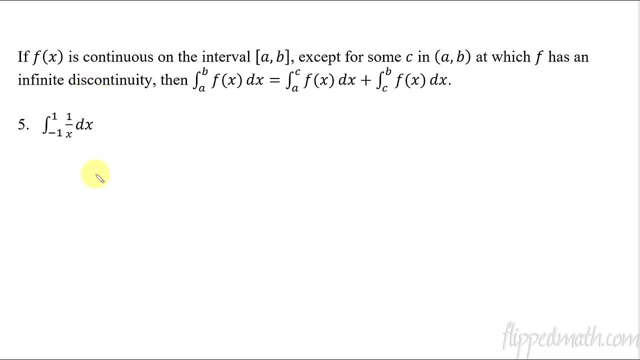 an infinite discontinuity, a vertical asymptote going on inside there. So here's a quick little. oh wait, I should show this. So what do we do? We take a and b and we split it up. we're going to go from a to c and then from c to 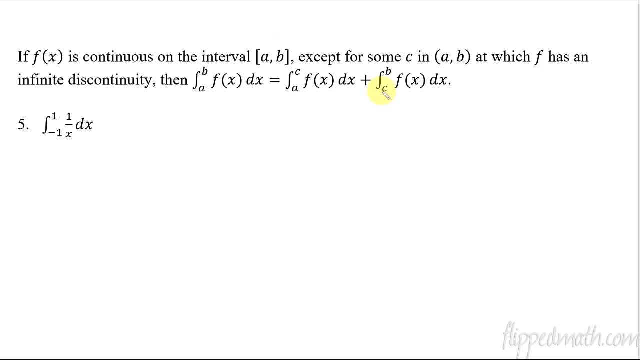 b. So we go from a to that vertical asymptote and then we go to the other side of the vertical asymptote and continue on until we get to b. So here's our example. We have a discontinuity at x equals 0, that's the problem. that's inside this interval. 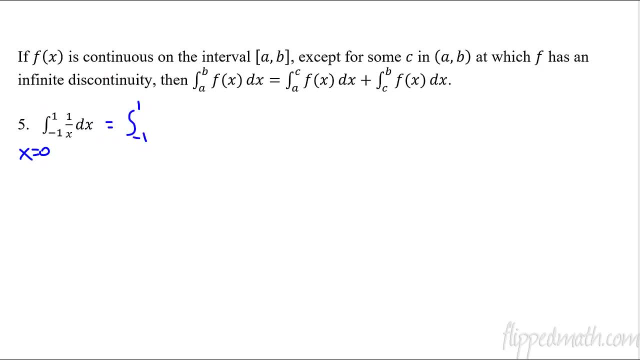 so I have to rewrite this as negative 1 to 0 of 1 over x, x with respect to x plus, and then we're going to go from negative 1,. no, I'm right, I'm messing this up, sorry. 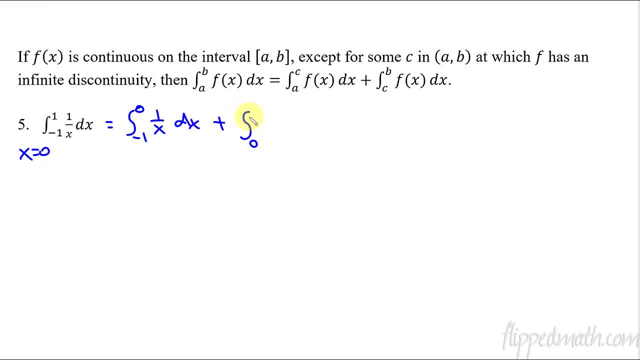 We've ended at 0, so we pick back up at 0,, start at 0, and then we go on until we finish the interval up to 1, of 1 over x with respect to x, So we can't actually evaluate it at 0. 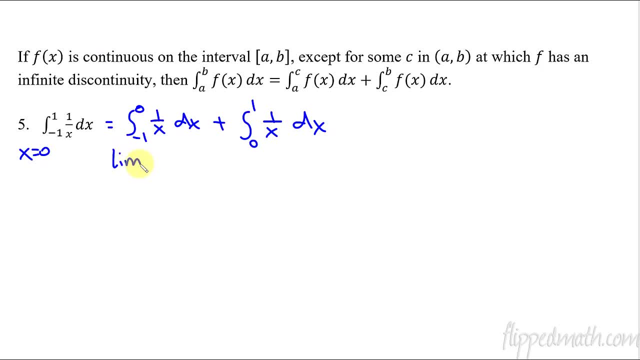 So this is where we have to do limit. So let's just set up the limits for the practice of it. we're going to say the limit of t is going to replace the 0. Okay, But what you have to think about is it the positive side or the negative side? 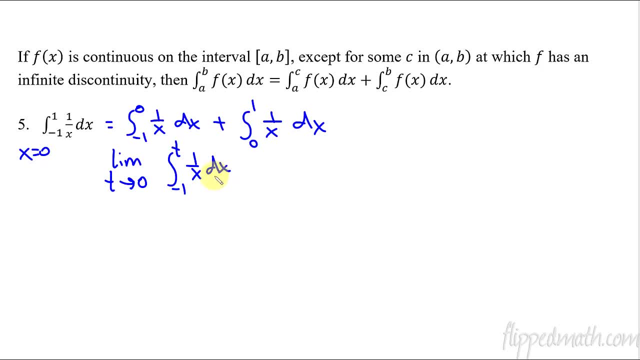 So we're going to go from negative 1 to t, of 1 over x with respect to x. So is it approaching 0 from the left or from the right? So if we're going from negative 1 to 0, we're approaching 0 from the left because we're 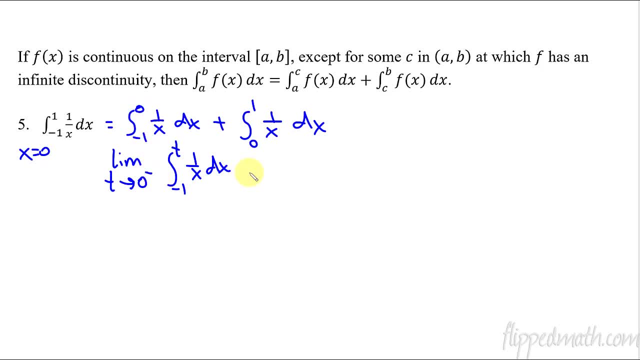 starting at negative 1 and going towards 0.. So that's how we know that: one Plus, and now let's do the limit as t approaches 0,. okay, I'm not going to put plus or minus yet, because I want you to think about this. 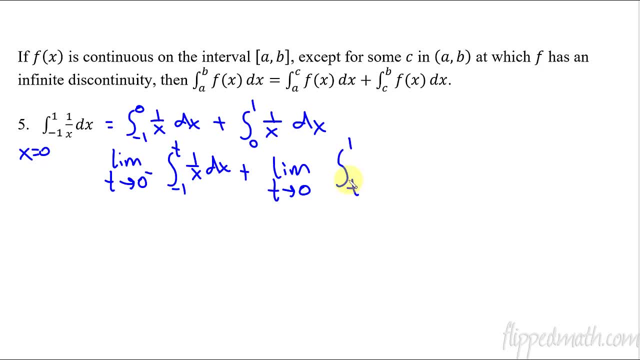 So 0 becomes the t, And then we're going up to 1.. So now we're starting at the t and going towards 1.. So we're approaching, we're having t approach 0 from the right side. So that's my 0, I'm approaching it from the right. 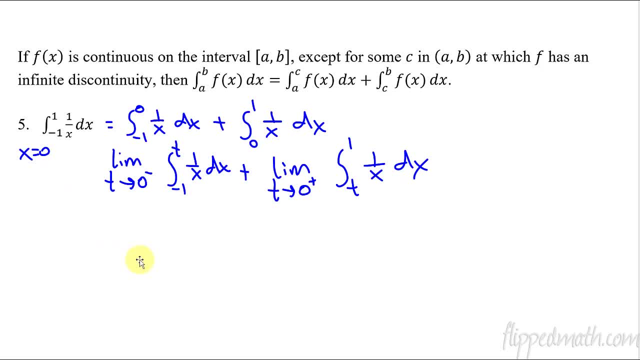 And then 1 over x with respect to x. All right, let's see what happens when we start taking the antiderivative. So I'm going to pause my recording and have the whole next line appear. So now that we have this line, I want you to realize what's going to happen. 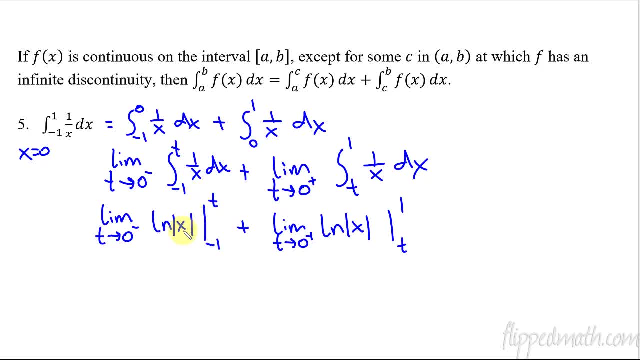 We're going to plug the t in subtract the 1. And the problem is that t is approaching 0. So if I'm going to end up with some type of natural log of t and that t is approaching 0, natural log of 0 doesn't exist. you can't do that.